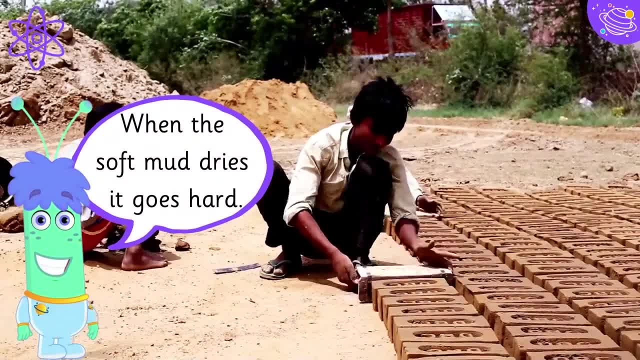 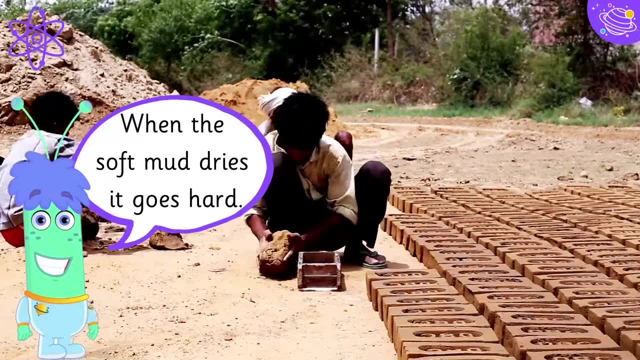 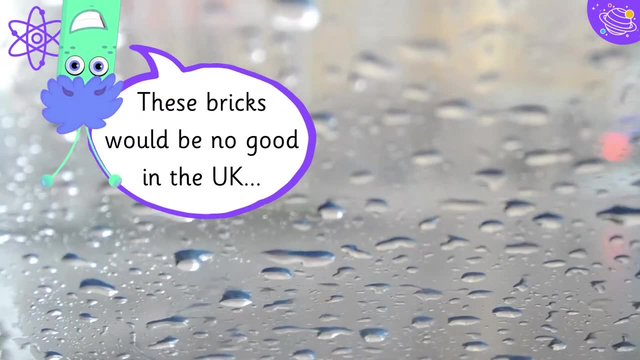 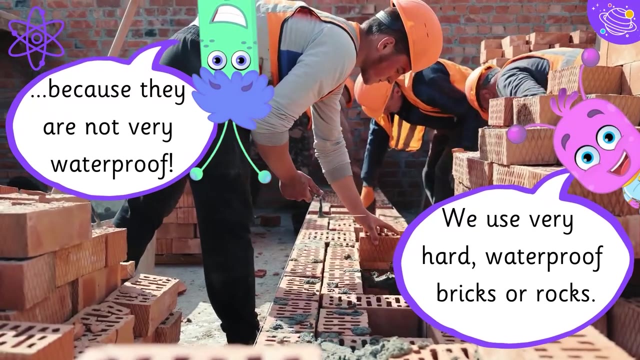 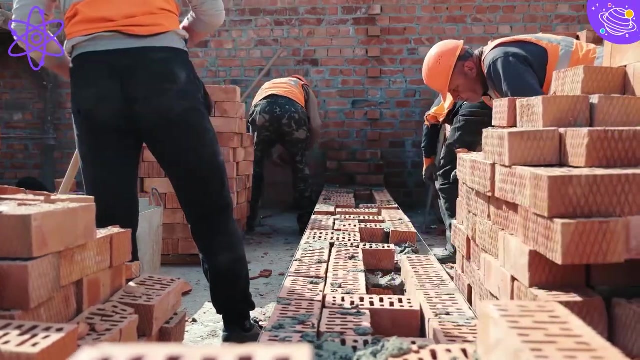 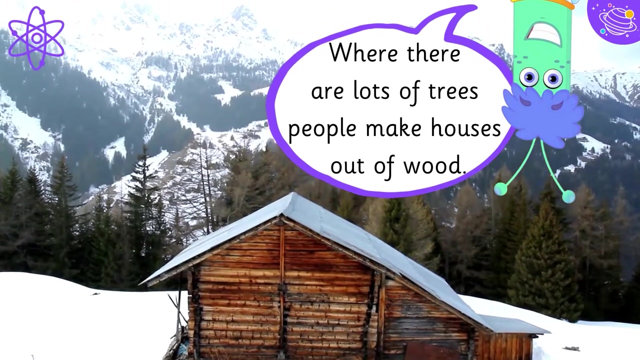 When the soft mud dries, it goes hard. These bricks would be no good in the UK Because they are not very waterproof. We use very hard waterproof bricks or rocks. Where there are lots of trees, people make houses out of wood. 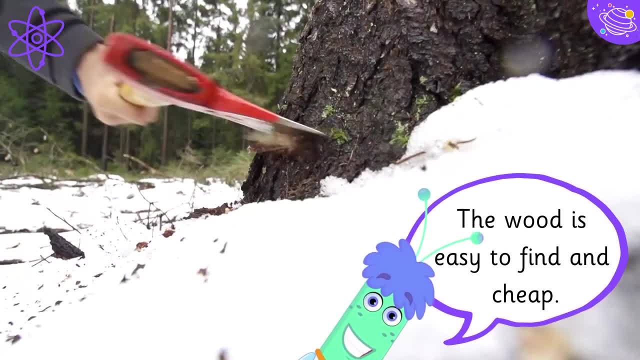 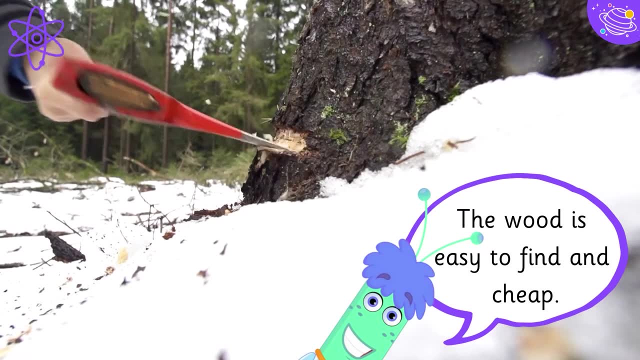 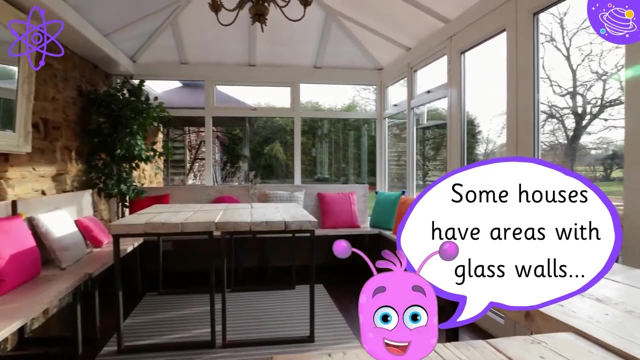 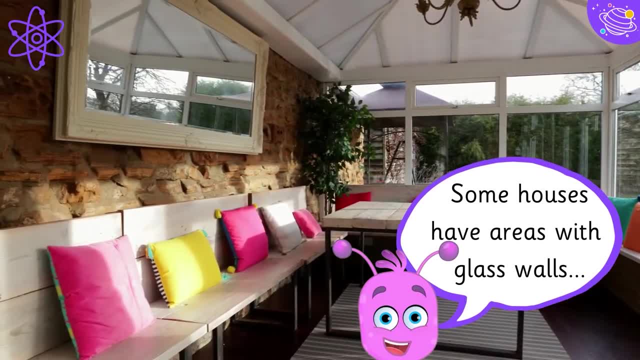 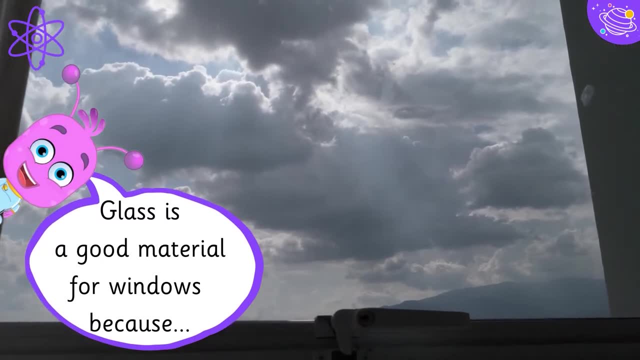 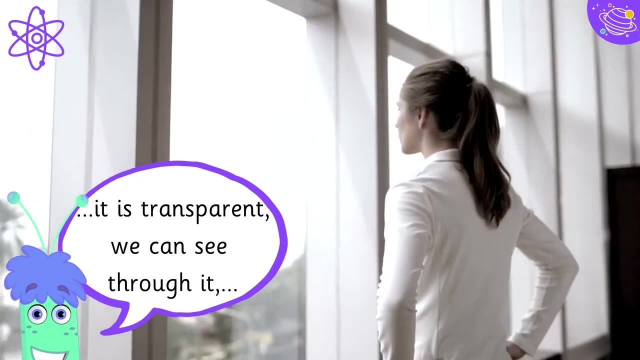 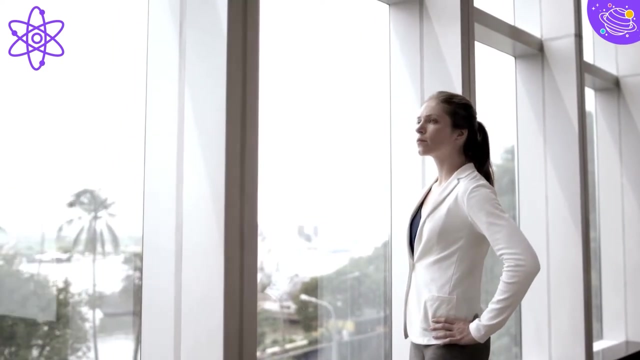 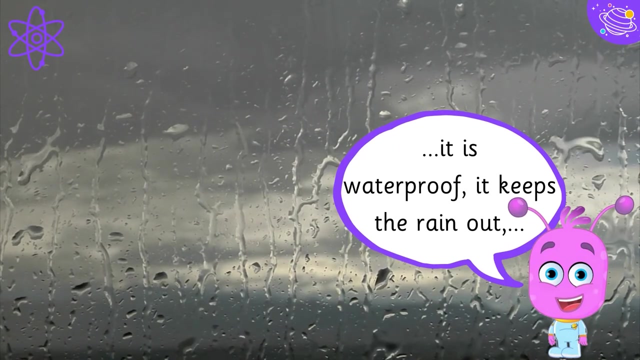 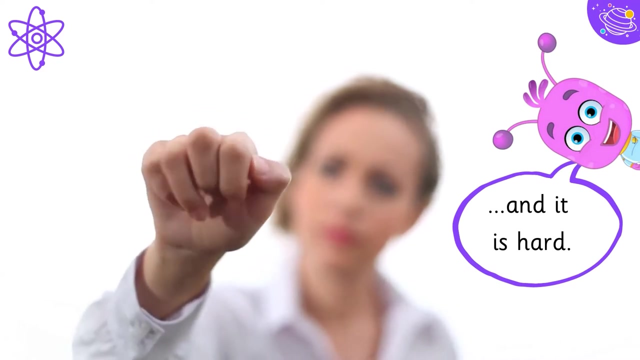 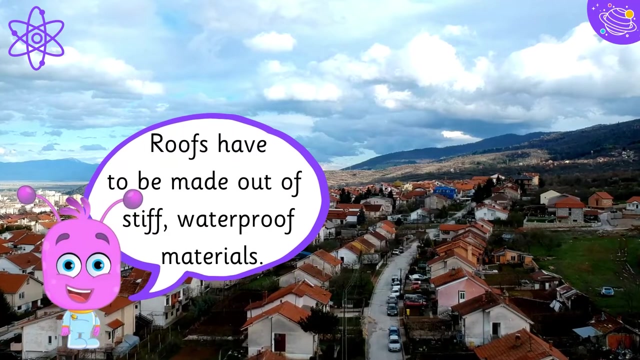 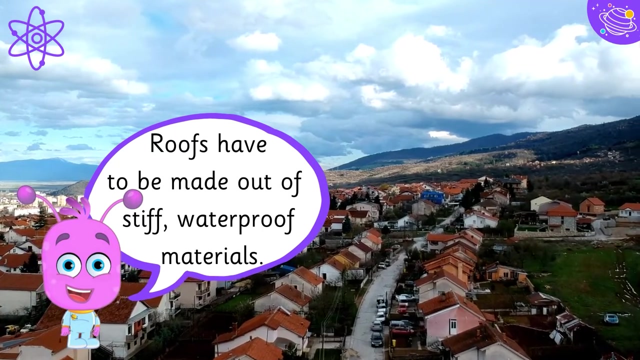 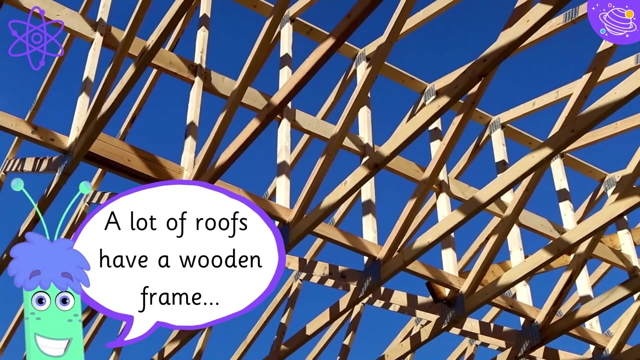 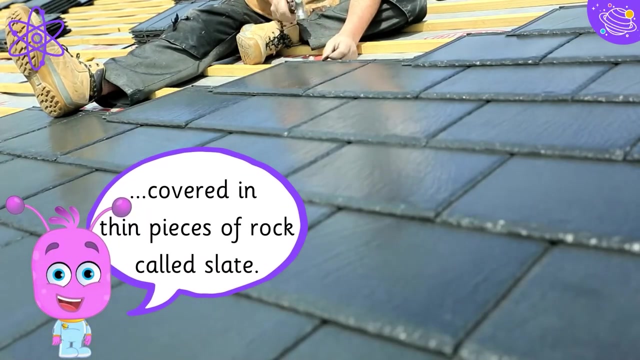 Glass is a good material for windows. because Glass is a good material for windows? because It is transparent. we can see through it. It is waterproof, it keeps the rain out And it is hard. Roofs have to be made out of stiff, waterproof materials. A lot of roofs have a wooden frame. 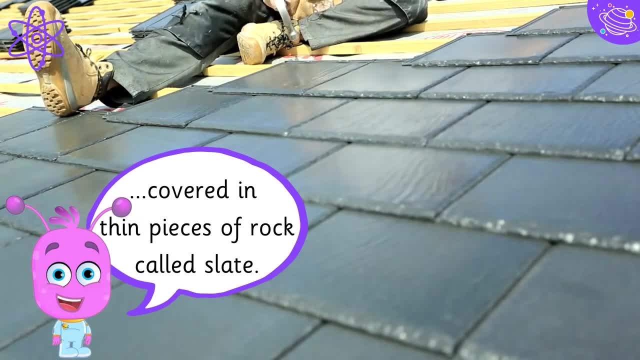 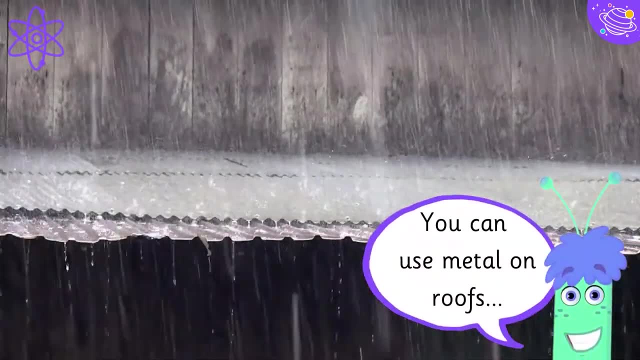 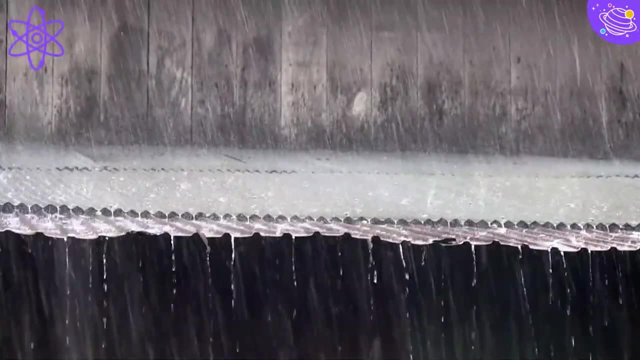 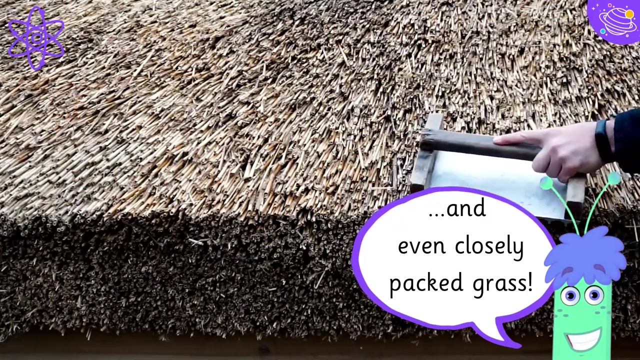 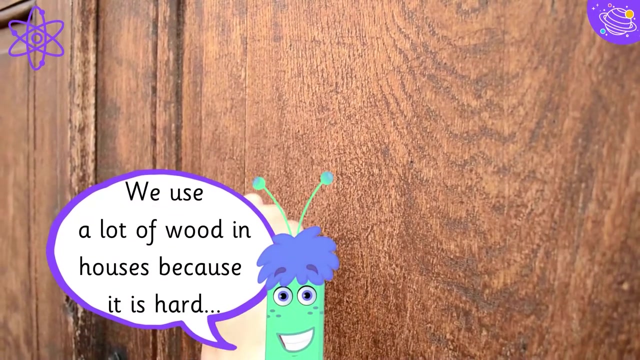 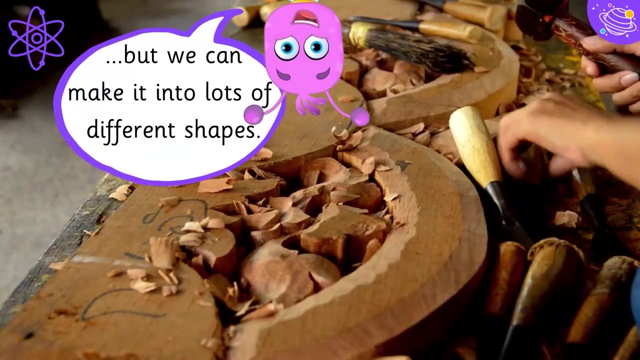 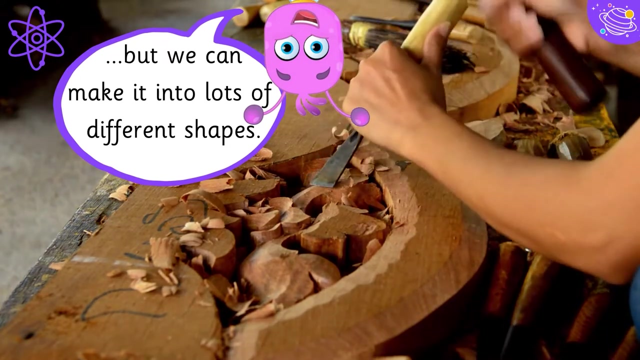 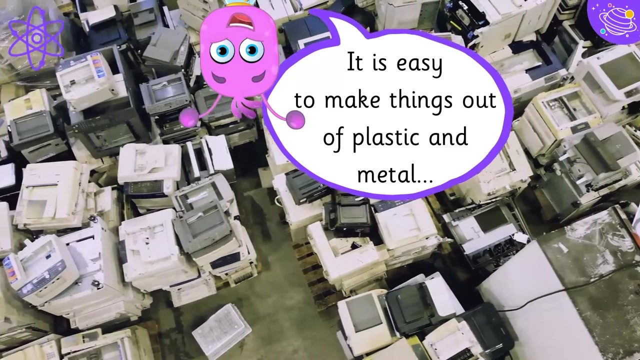 With in thin pieces of rock called slate. You can use metal on roofs And even closely packed grass. We use a lot of wood in houses because it is hard, But we can make it into lots of different shapes. It is easy to make things out of plastic and metal.